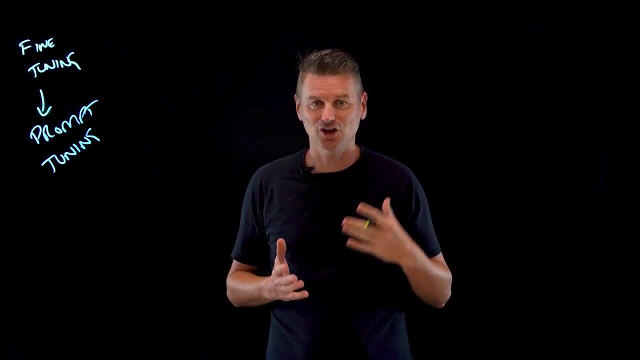 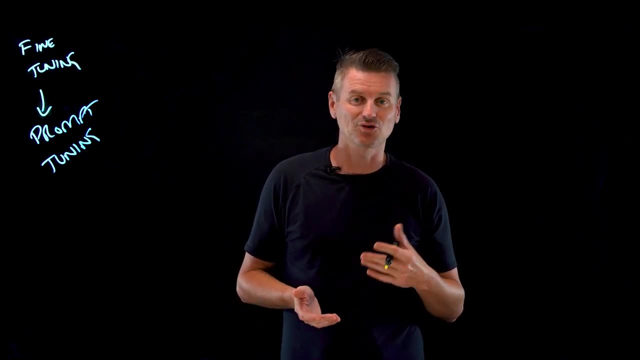 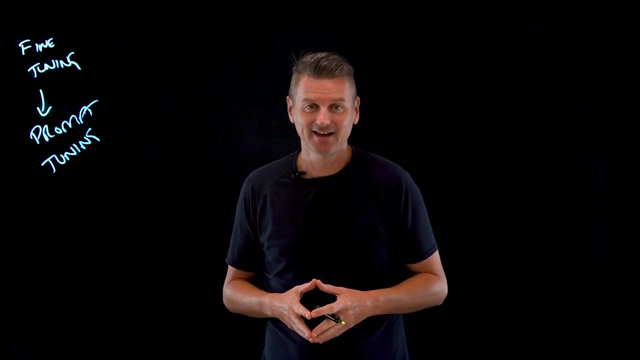 like we have to do with fine tuning. In prompt tuning, the best cues or front-end prompts are fed to your AI model to give it task-specific context. The prompts can be extra words introduced by a human or, more commonly, an AI-generated number introduced into the model's embedding layer to guide the 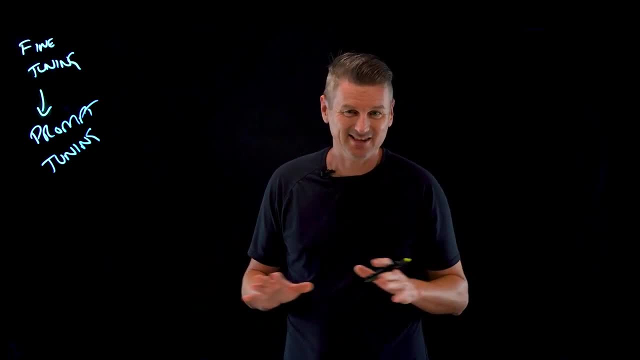 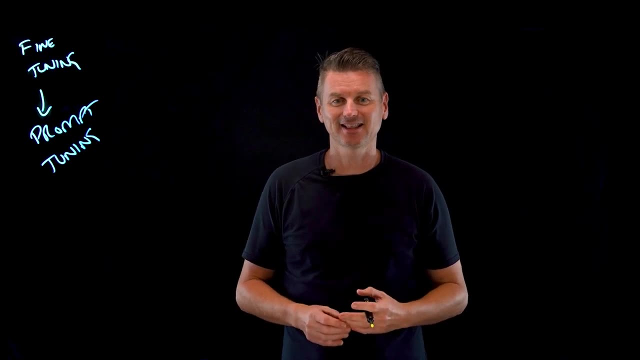 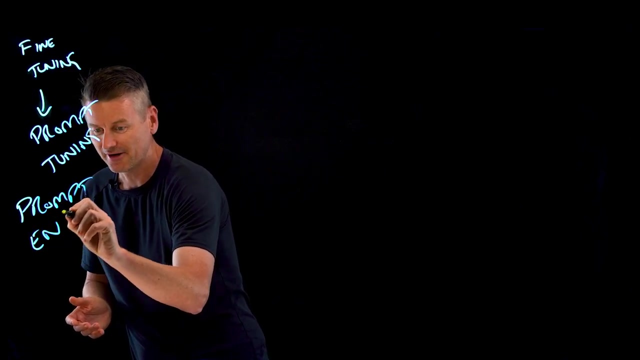 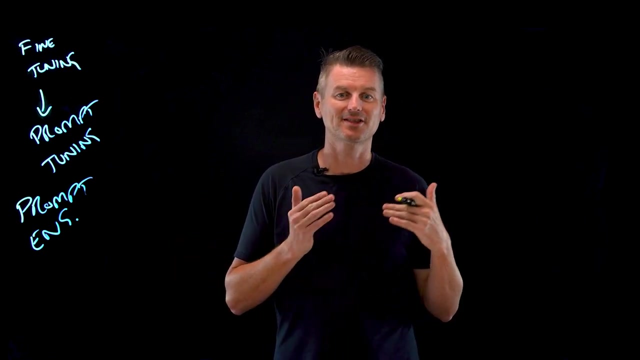 model towards a desired decision or prediction. Now, if all this sounds a little bit familiar- using prompts to guide the output of an LLM- that's because it most certainly is. That is an example of something else called prompt engineering. Now, prompt engineering is the task of developing prompts that guide an LLM to perform specialized 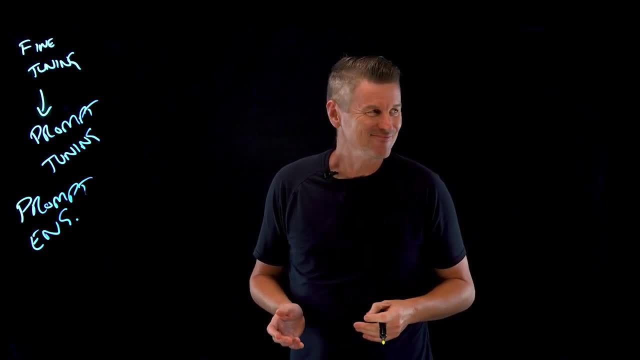 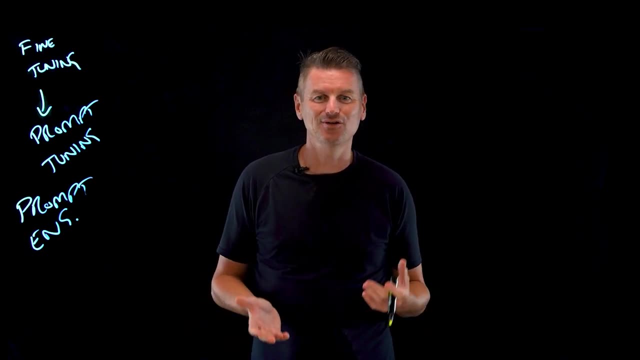 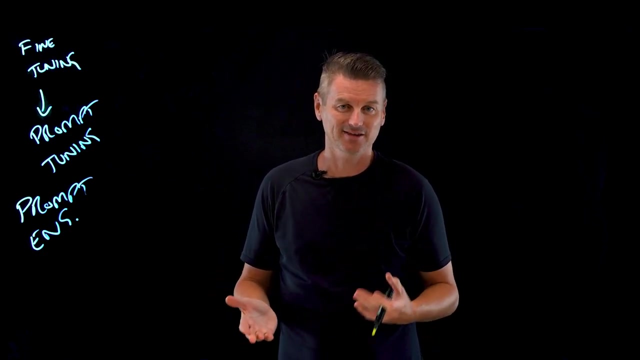 tasks. Honestly, it sounds like a lot of fun. I think I'd quite like to be a prompt engineer one day. So if I want my LLM to specialize as an English to French language translator, I might engineer a prompt to do so. So my prompt might start with, let's say, translate, And we want to. 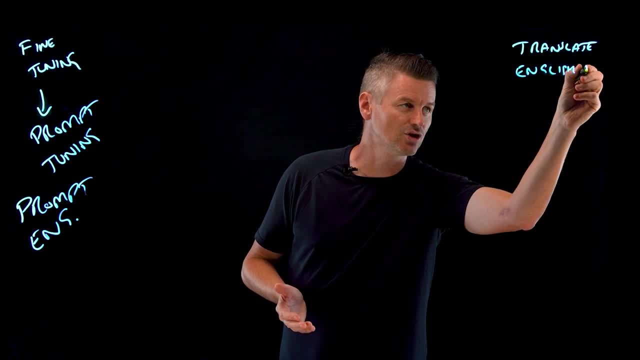 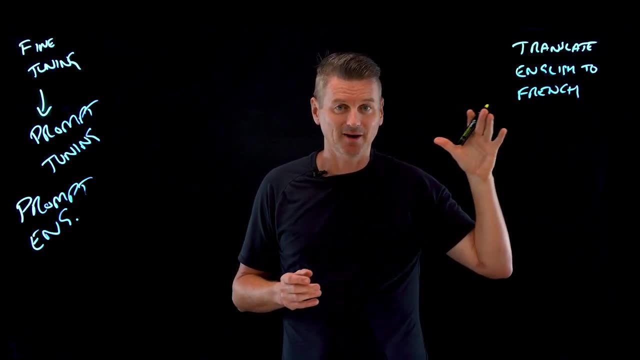 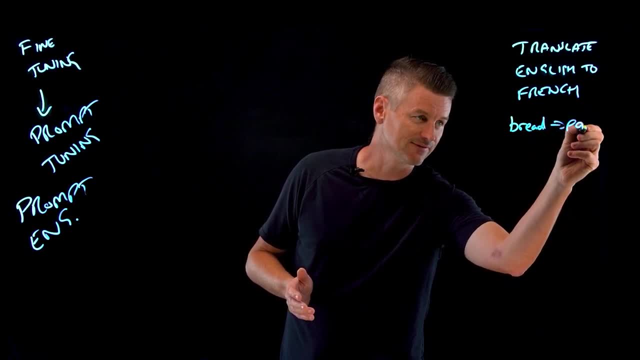 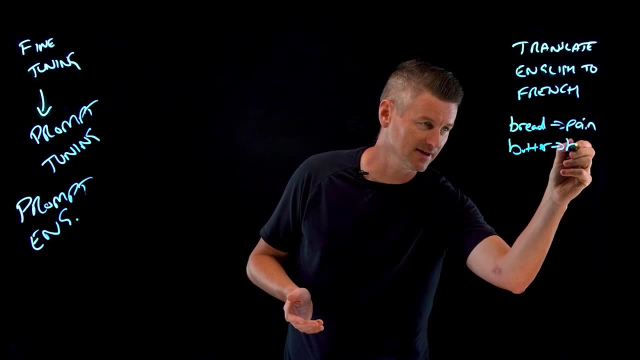 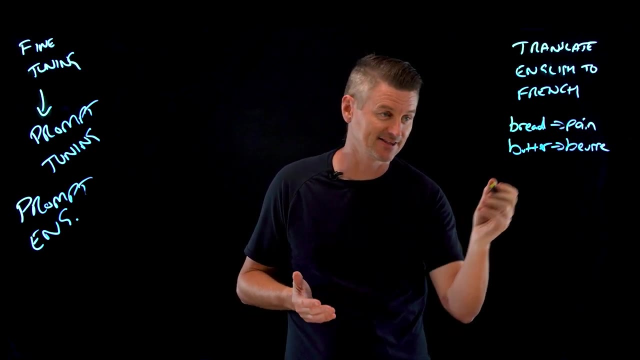 So here's the English word bread into the French word pan. That's one shot example. Let's add another Butter. We're going to turn that into beer, And then the next part of the prompt is: I'm going to add the word that I want it to translate next, So cheese. And that's it Now prompts. 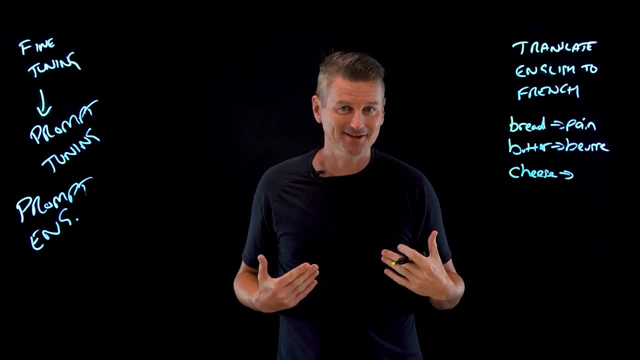 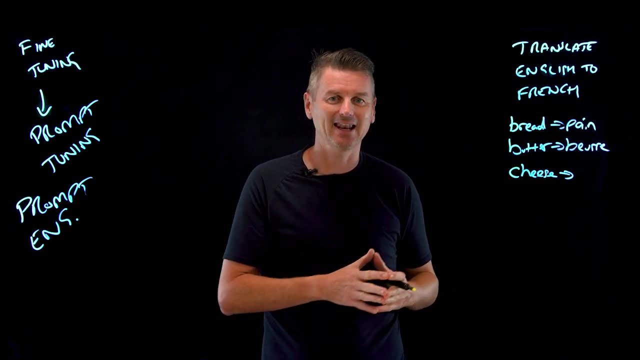 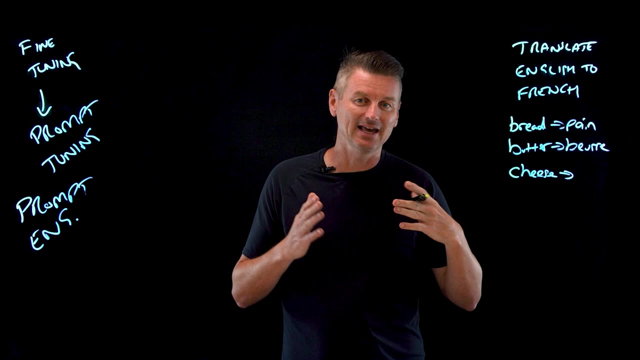 like this, written by a human me, Mr Wannabe, prompt engineer himself. they prime the model to retrieve the appropriate response from the LLM's vast memory, In this case specifically for other words in French, And the model's output is its prediction. What is this model going to output? 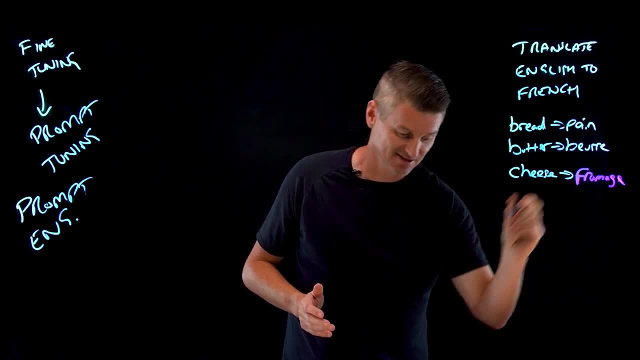 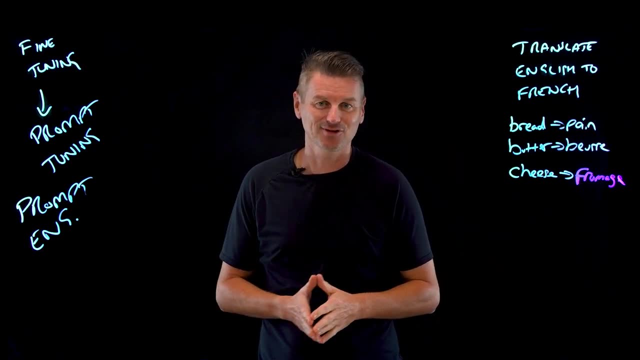 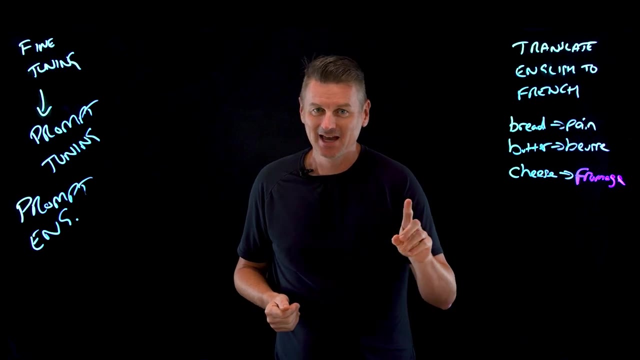 Fromage That worked. We've used prompt engineering to train a model to perform a specialized task with just a single prompt introduced at inference time without needing the model to be retrained. But if the task is more complex than this, it may require dozens of. 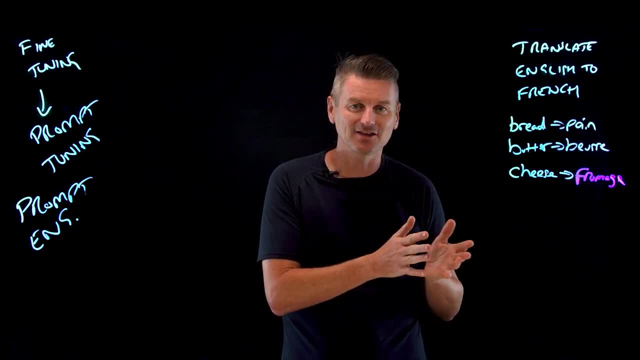 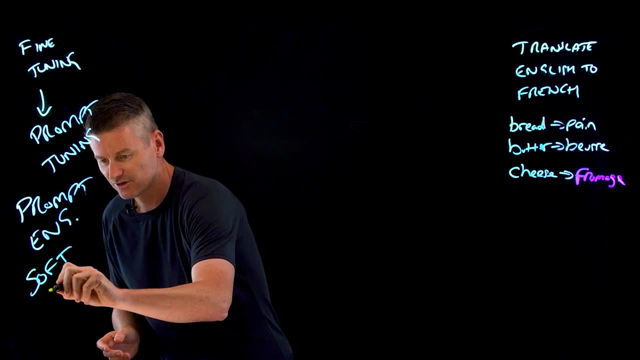 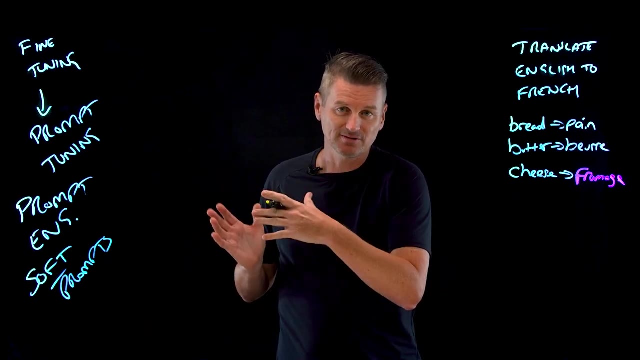 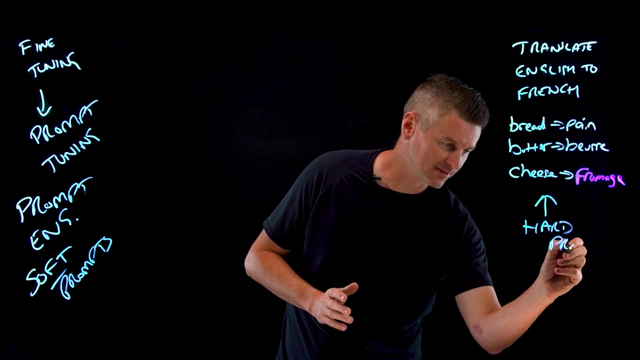 these prompts, And so these handcrafted prompts have begun to be replaced by AI designated prompts, Known as soft prompts. Now, soft prompts have been shown to outperform human engineered prompts, which we can know now as hard prompts. These were hard coded by a human. This is not good news for 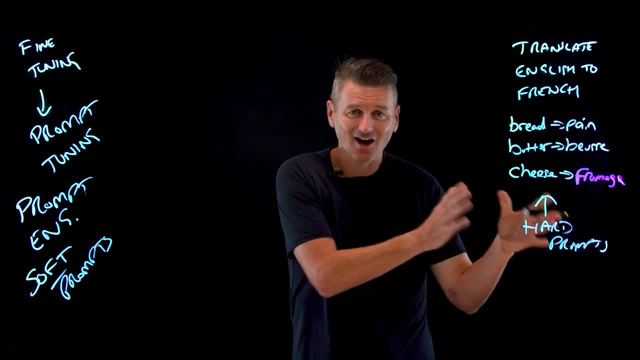 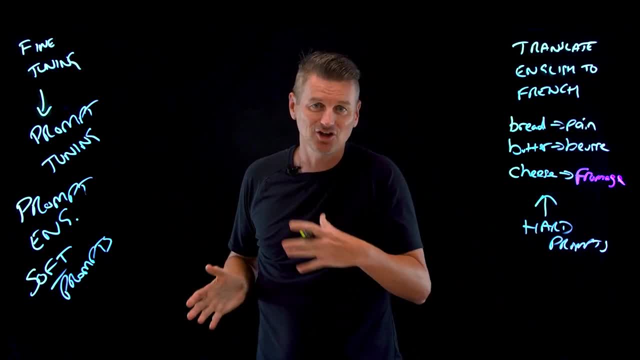 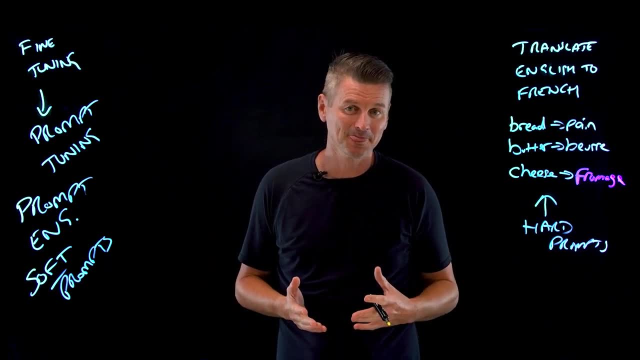 They're used in prompts that are not soft prompts And they are unrecognizable to the human eye. Each prompt consists of an embedding or strings of numbers that distill knowledge from the larger model, And these soft prompts can be high level or task specific and act as a substitute for 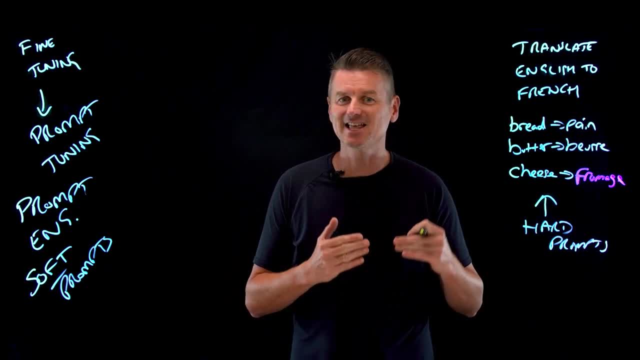 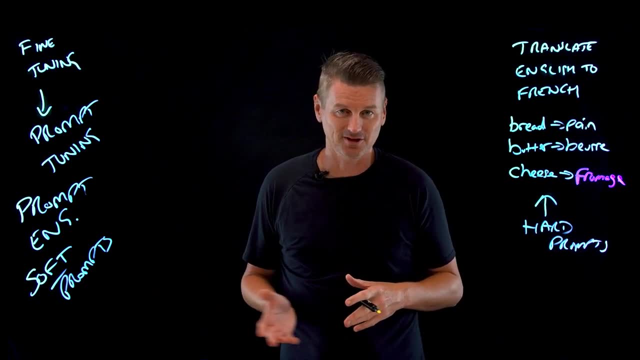 additional training data and incredibly effective in guiding the model towards the desired output. But do keep in mind that one drawback of prompt tuning and soft prompts in general is its lack of interpretability, And that's because they're not the same as soft prompts. They're not the same as soft. prompts, And that's because they're not the same as soft prompts. They're not the same as soft prompts, And that's because they're not the same as soft prompts. They're not the same as soft prompts. That means that the AI discovers: 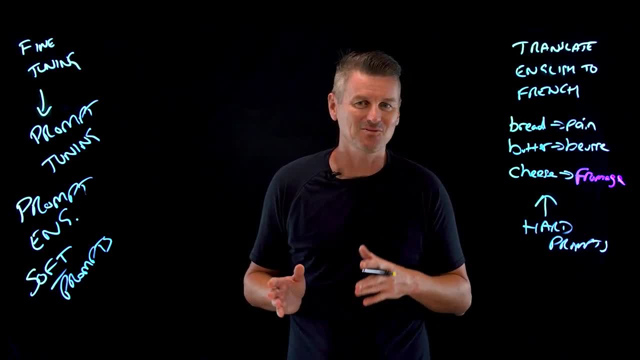 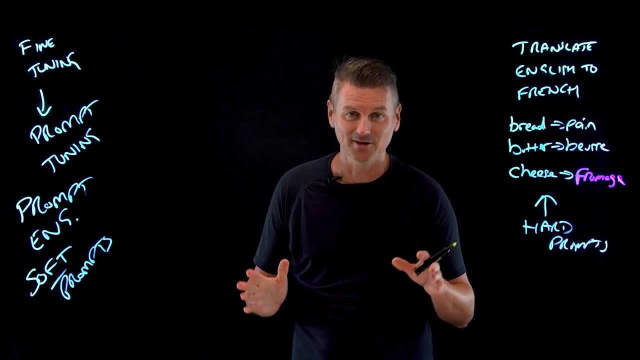 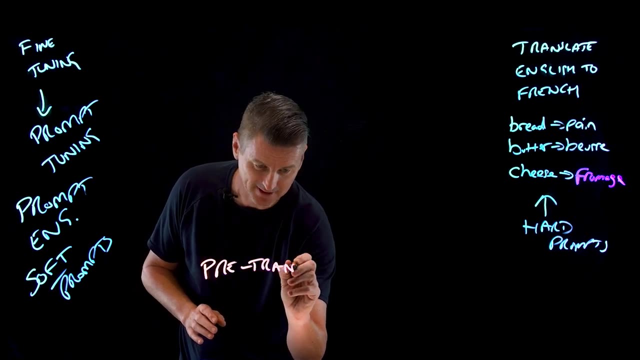 prompts optimized for a given task, but it often can't explain why it chose those embeddings. Like deep learning models themselves, soft prompts are opaque, All right. So let's consider: we have here a pre-trained model, So this might be a large language model, something like that. 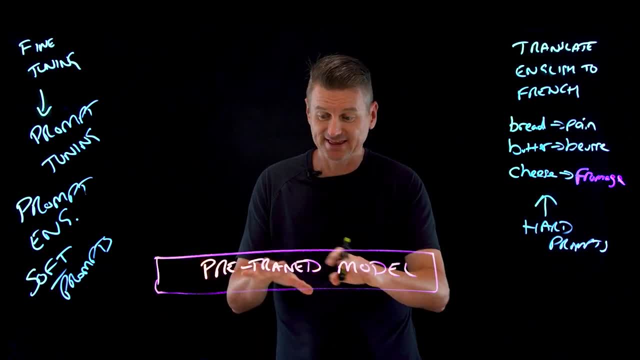 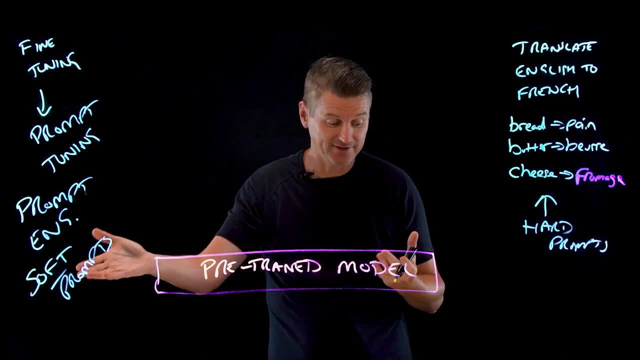 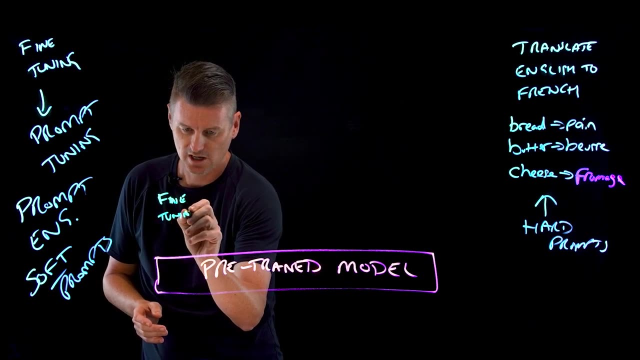 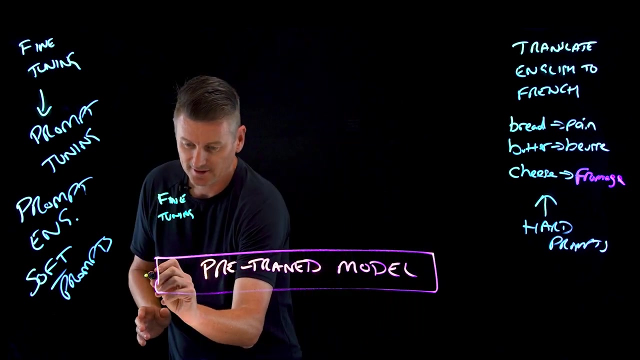 Okay, Now let's consider three options for prompt tuning. So the first one is for tailoring this pre-trained model for specialization. I'm going to talk about the three that we've covered here. So first of all, fine tuning, Fine tuning. So with fine tuning, we take this pre-trained model and we supplement it. We supplement. 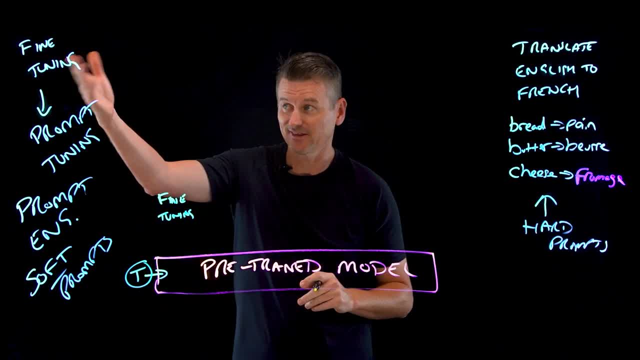 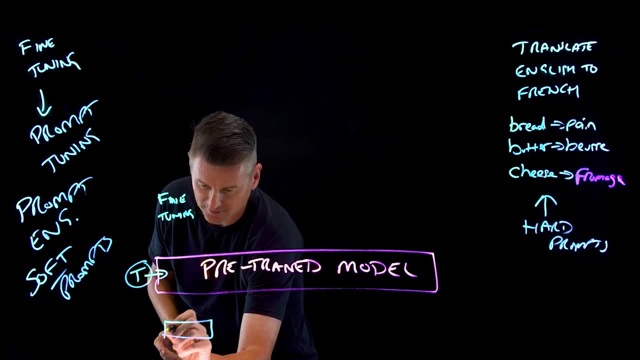 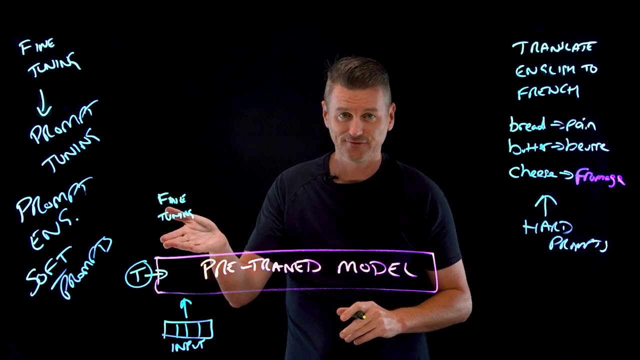 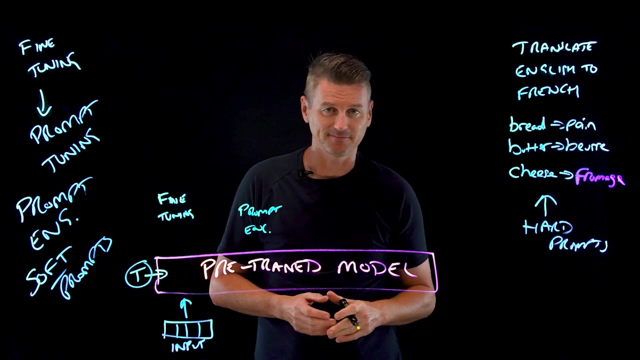 it specifically with tunable examples. These are the thousands of examples that I talked about right at the beginning. Once we've done that, We can then provide our input data into the model, and it should now be able to perform our specialization. So that's fine tuning. What about prompt engineering? How is that different? 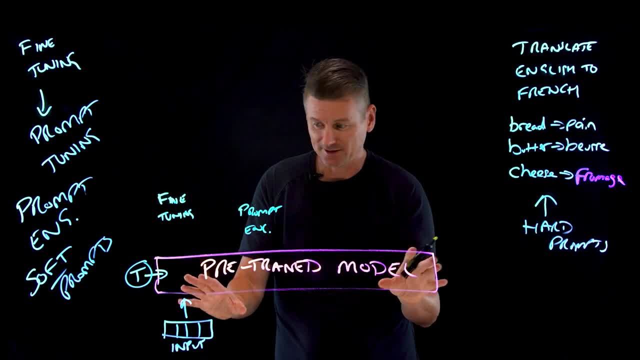 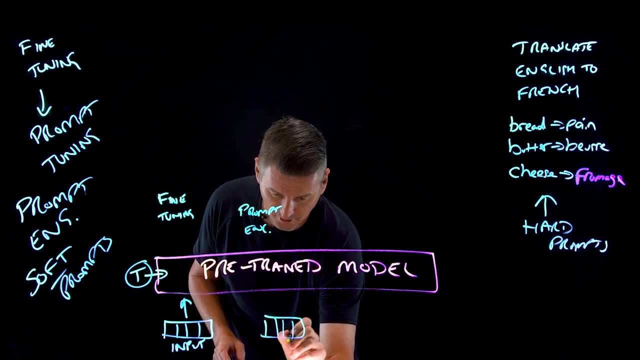 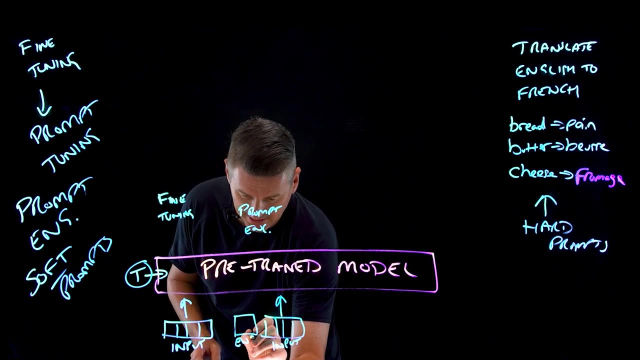 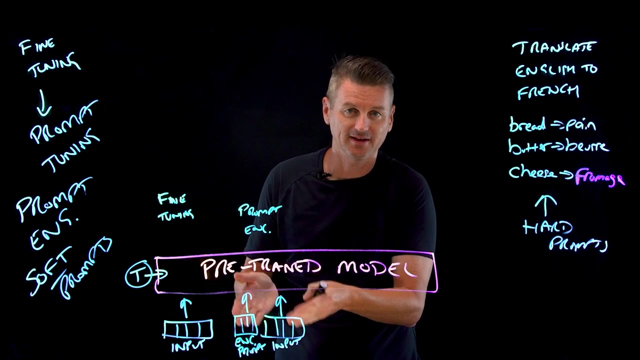 But with prompt engineering we take the model as it is- We haven't tuned it- and then we add in an additional prompt. So we have our input prompt, but we also add into that input prompt an engineered prompt which sits in front of it. So we effectively provide two prompts here for. 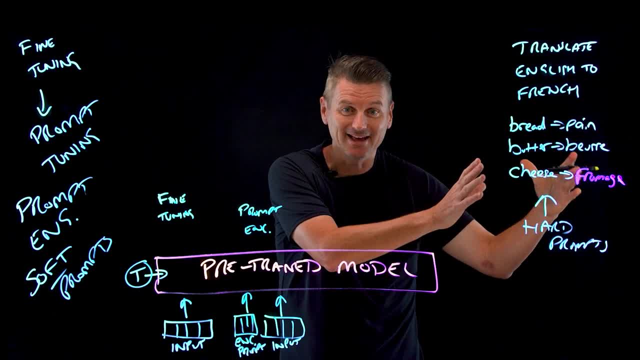 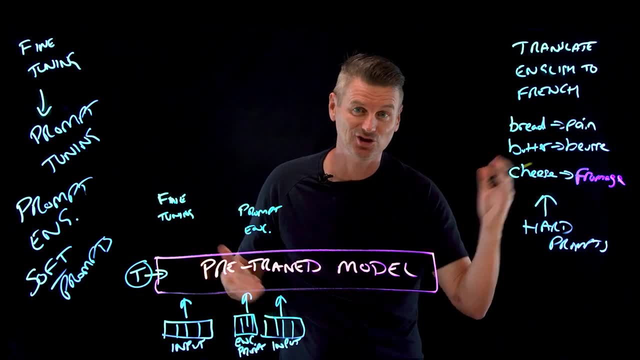 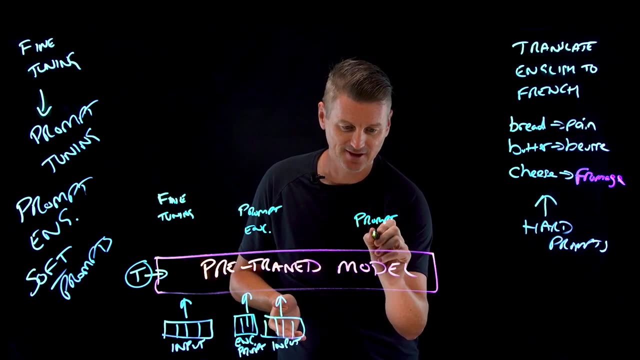 the specialization That's. that's what we did with our language translator. So we provided this pre-written engineered prompt and then we provided our input, which was cheese. So that's it, prompt engineering. What about prompt tuning? How is that different? Well, with prompt tuning, 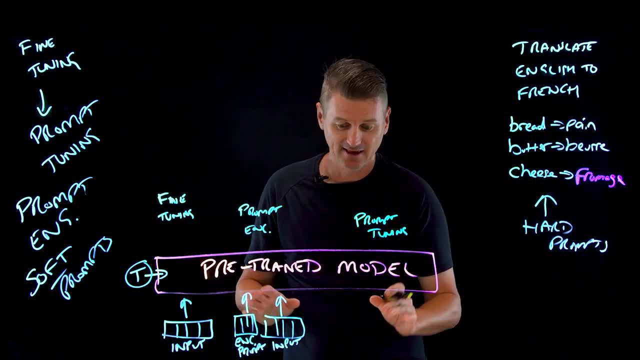 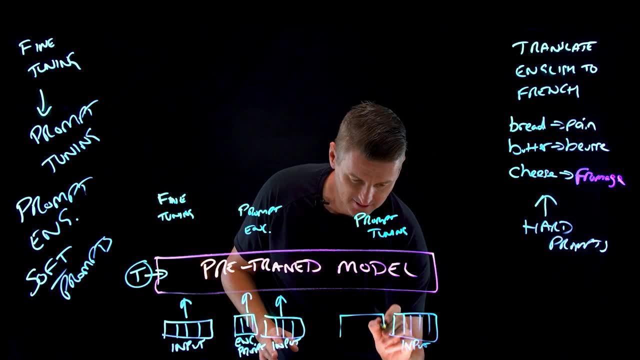 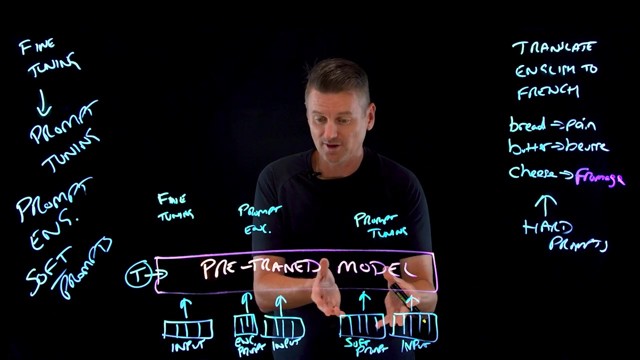 again, we use the pre-trained model as it is and we again provide an input, But we also provide something in front of that input, and that is the tunable soft prompt that is generated by the AI itself, And it's the combination of these two things that allow us to use the model in a 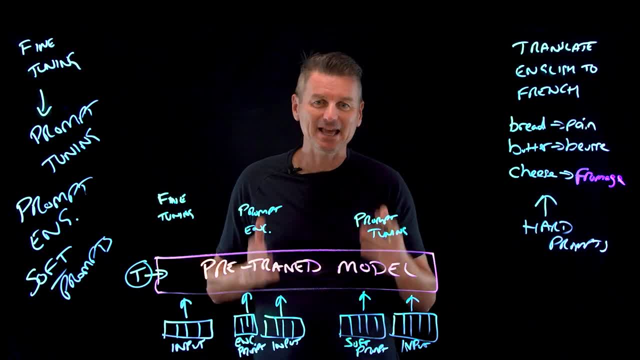 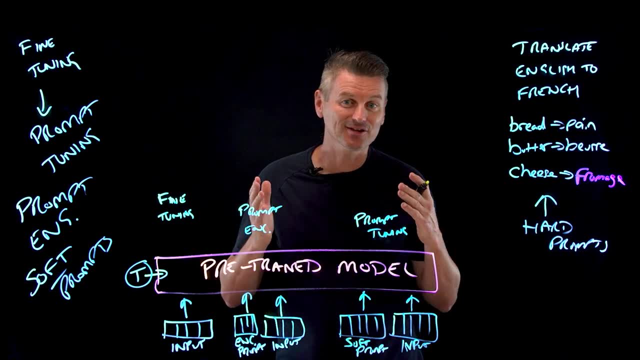 specialized way. Prompt tuning is proving to be a game changer in a variety of areas. For instance, in multi-task learning, where models need to quickly switch between tasks. researchers are finding ways to create universal prompts that can be easily recycled. Techniques like multi-task 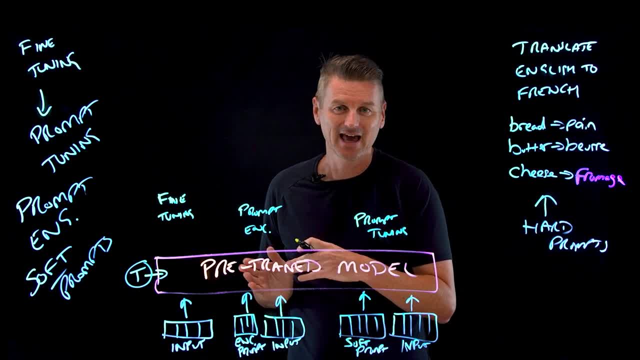 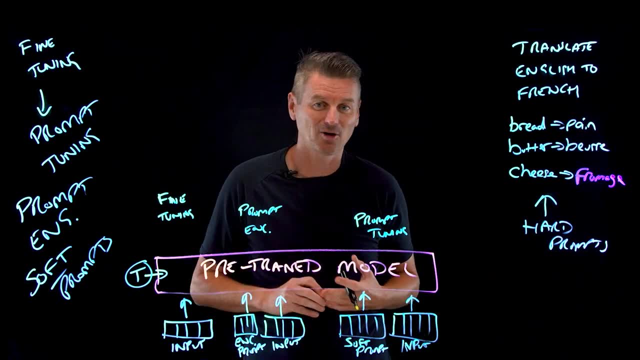 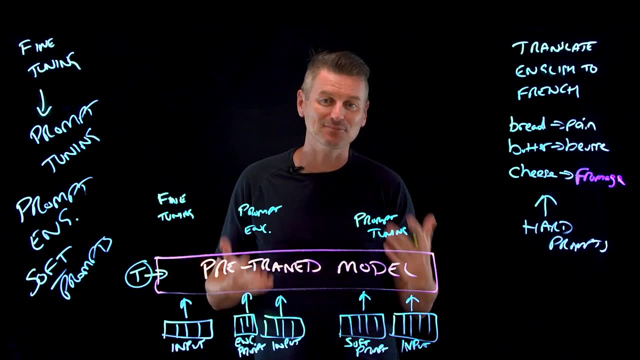 prompt tuning allow the model to be adapted swiftly and for a fraction of the cost of retraining. Prompt tuning is also showing promise in the field of continual learning, where AI models need to learn new tasks and concepts without forgetting the old ones. Essentially, prompt tuning allows you to adapt your model to specialized tasks.